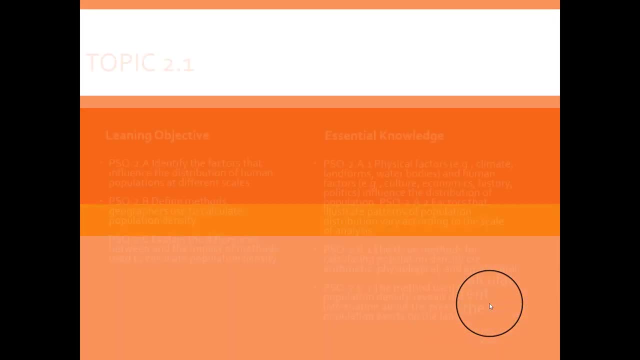 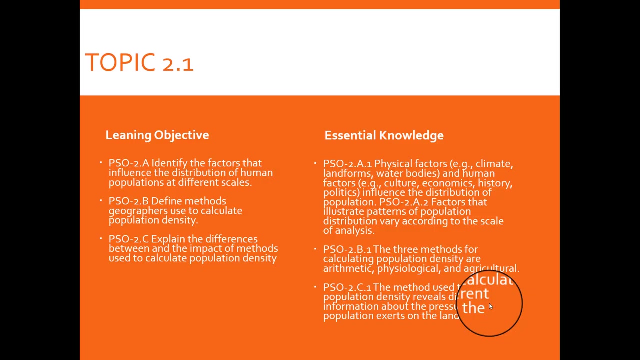 Across the planet, right, Okay, let's go. So this is our learning objectives and our essential knowledge that we're going to be going through in this lesson. However, I want to just put it in layman's terms for you. 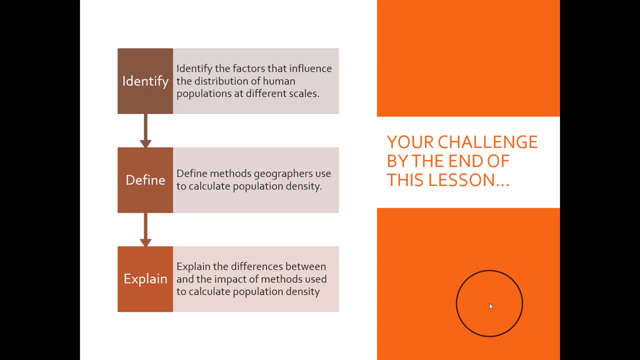 So your challenge for this particular lesson is to identify the factors that influence distribution of human populations at different scales, define the methods geographers use to calculate population and then be able to explain the differences between the population densities and the impact of the methods used to calculate population density. 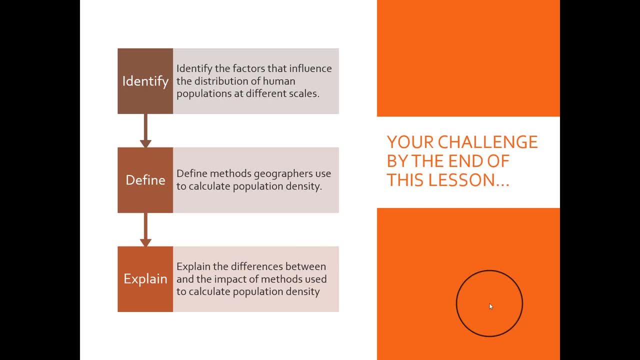 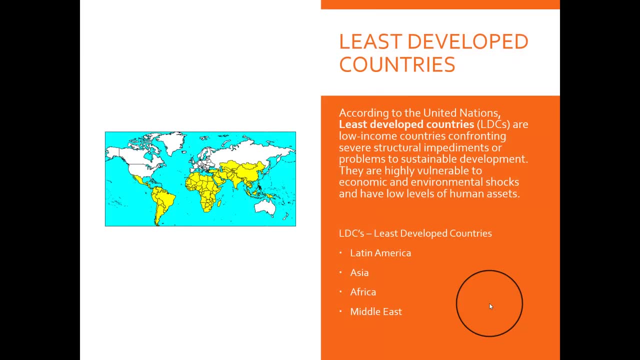 So you have a big challenge for this lesson, but I think you'll be able to do it by the time we're finished. Okay Alright, So first off, we need to know about countries. So there are least-known countries. 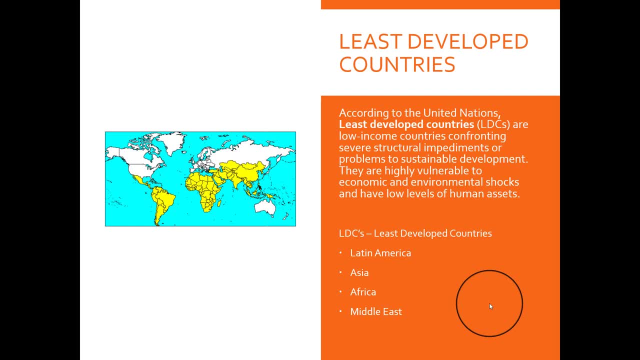 There are least-developed countries And, according to the United Nations, least-developed countries are low-income countries confronted with severe structural impediments or problems to sustain their development. Okay, Meaning that they have a very hard time upholding their society because of low-income status. 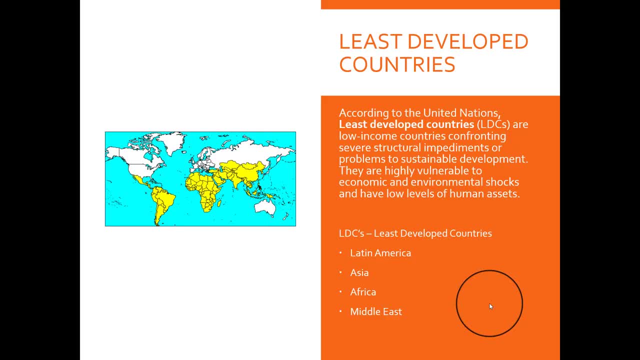 Okay. They're very vulnerable to economic and environmental shocks and have low levels of human assets. Human assets means anything that would help to propel the society economically speaking. Okay, So any resources or anything like that that would help to propel the society economically. 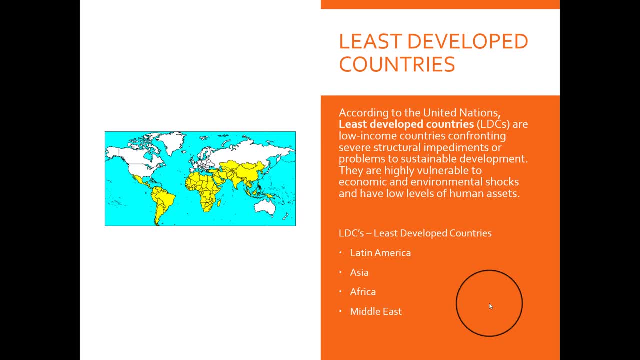 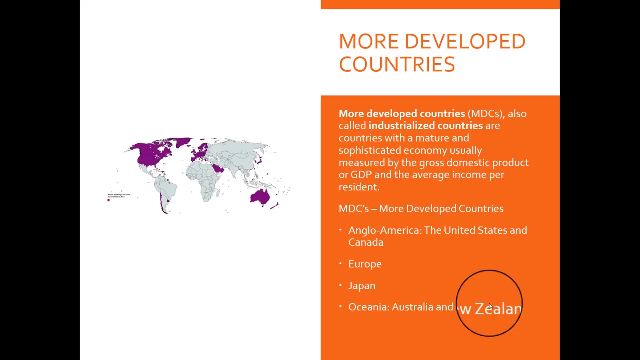 And examples of LCDs, or least-developed countries are Latin America, Asia, Africa and the Middle East. Okay, And now we have more-developed countries. More-developed countries, or MDCs, are also called industrialized countries, And those countries have a mature and sophisticated economy, which is usually measured by the gross domestic product, or the GDP, and the average of the income per resident. 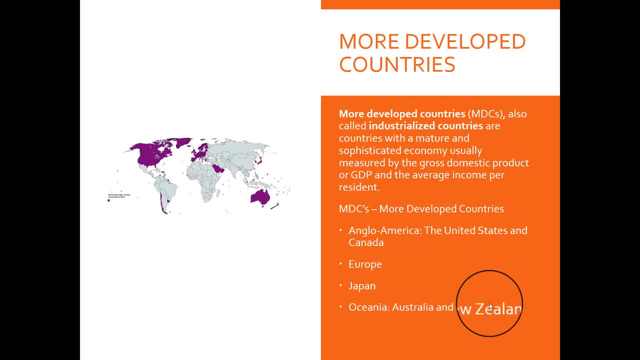 So, in this case, more-developed countries have a highly sophisticated economic system, And that economic system and the resources that they need, The resources that they have, truly support and advance the society so that it gets bigger and more grander Right. 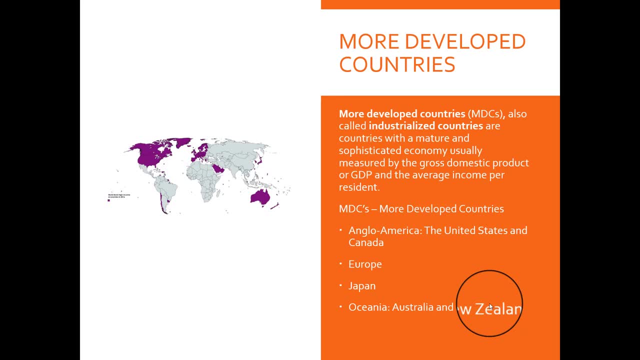 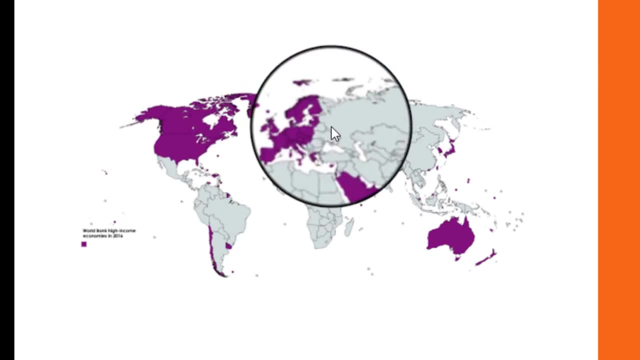 So MDCs. Some examples of MDCs are the United States and Canada and Anglo-America, as you see here in this map: Right Europe, Japan and parts of Oceania. Right, Australia and New Zealand: Parts of Oceania. 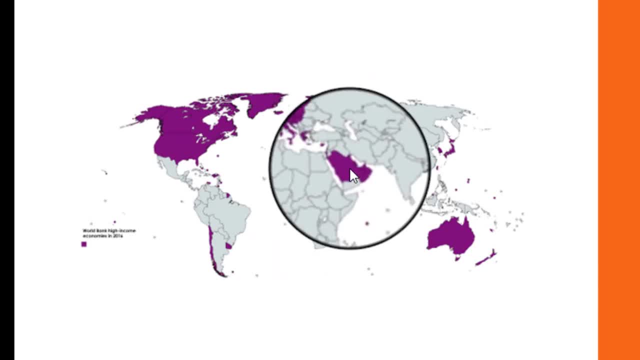 And there's also some parts of the Middle East as well. Okay, Not entirely. The entire Middle East is LCD, because there are certain places like Saudi Arabia that's very rich in oil deposits and oil distribution And that's where we get our resources for our gas. 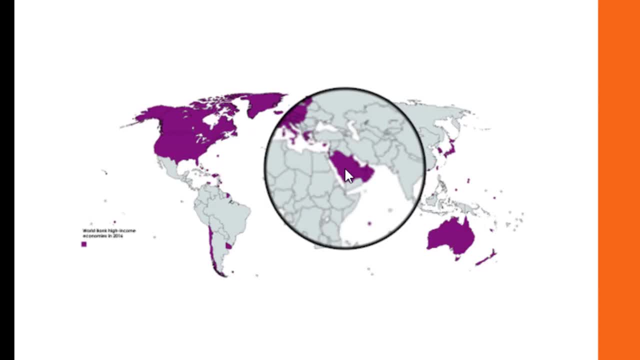 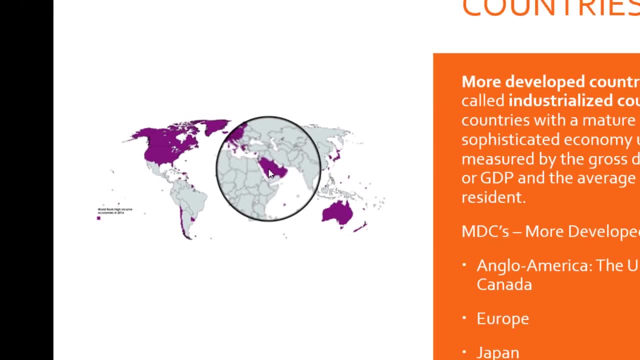 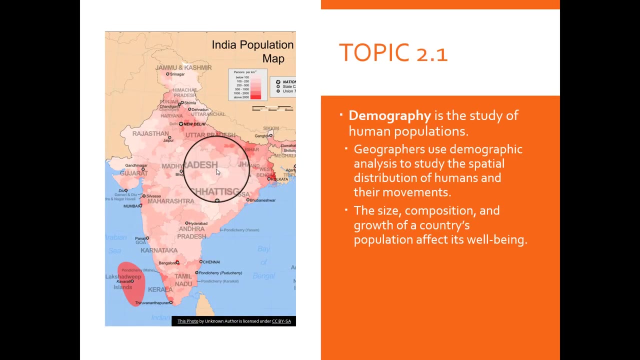 So not all countries in the Middle East are LCDs. In this case, Saudi Arabia is an MCD Right, Alright, So let's continue. Alright, So demography is the study of human populations. Okay, And basically, geographers use this information, or demographic analysis, to study the distribution of humans over the Earth and how we move as well. 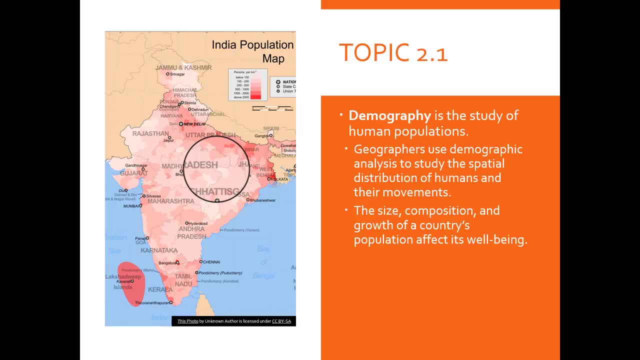 Okay, So the size and the composition and the growth of a country's population definitely affects its well-being. So, depending on how big it is, the size, How it's composed And also how it is growing in terms of whether it is an LCD or an MCD, 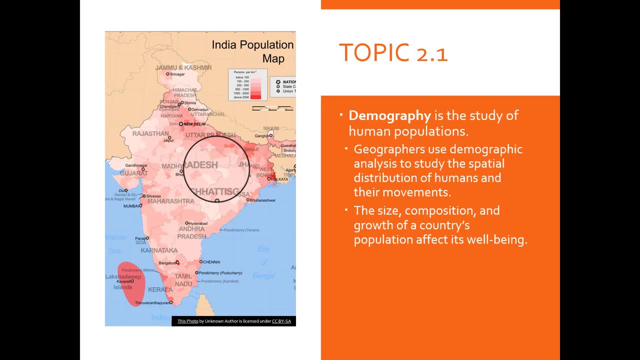 It depends on the well-being and the survival of that particular country. Okay, So, as you see here in this map, this map kind of shows the population of India And there's certain places that's very close to the capitals, Right. 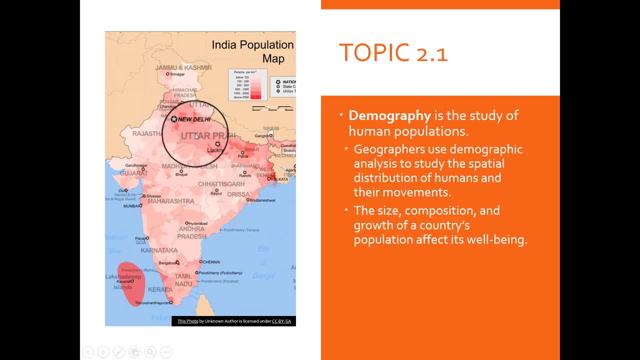 That are highly dense, Okay, And there's a lot of people per person per kilometer in those certain areas, Right? So it kind of lets us know what the demography is in that area in terms of how people take up space in those areas or in those places. 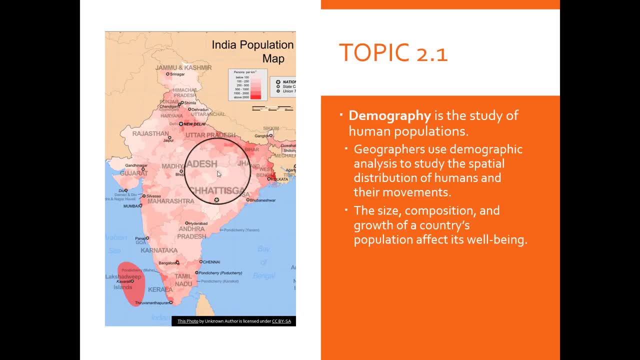 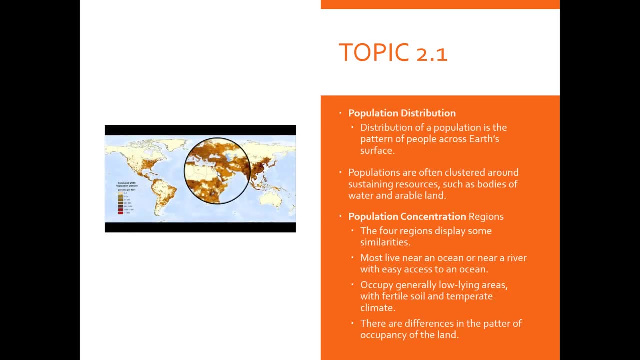 And kind of asking the question: why did they take up space in those areas? Alright, So population distribution is the distribution of a population in this pattern, across the pattern of people across the earth. Okay, So basically we're looking at the pattern of how many people are placed or living in certain places on the earth. 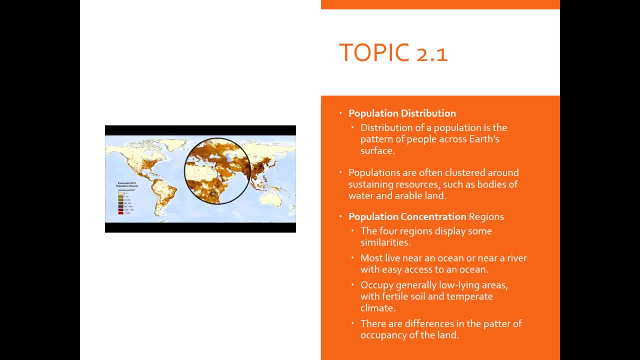 Okay, And usually populations are often clustered across the earth, Clustered or concentrated near things that are sustainable, like water and farmable land. Areable means farmable, Okay, So population concentration regions. there's usually four regions that display the same similarities. 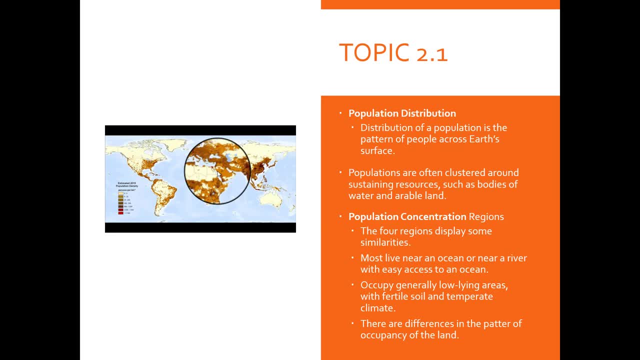 It's usually near some form of water or river or some kind of easy access to the ocean. Okay, Usually there's some form of fertile soil And there's also some type of climate that is temperable, Meaning that you can, it's livable. 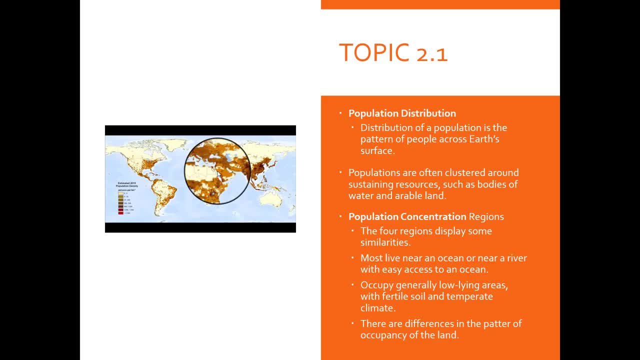 It's not too hot, It's not too cold, You know, and it's not too warm, Those kind of things, Right. And there's differences in the patterns of the occupancy on the land itself. So it's not just that it's highly concentrated in all the areas. 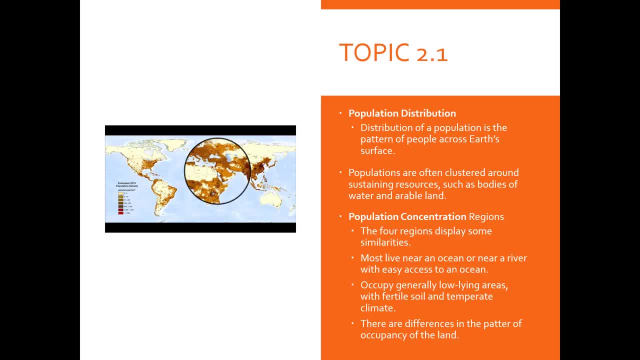 There may be spots where it's sparse- And sparse means that there's not that much- And then there's areas where it's highly concentrated. As you see here in the map, there's certain areas, especially in India and in China, where it's highly concentrated. 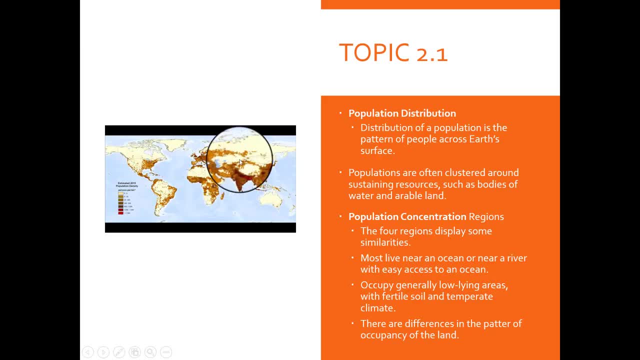 Right, And some places in Europe And then other places where it's not so concentrated at all. Right, There's barely barely anybody, Okay, So that's called population distribution, Alright. So if we look at population distribution, 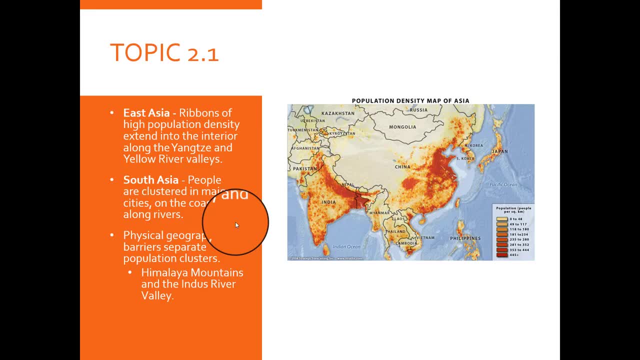 Some of the places that are highly, highly, highly dense in population are East Asia and South Asia, And the reason for that being is that a lot of this area, historically speaking, like in India and in these areas here, this is what was called the Fertile Crescent. 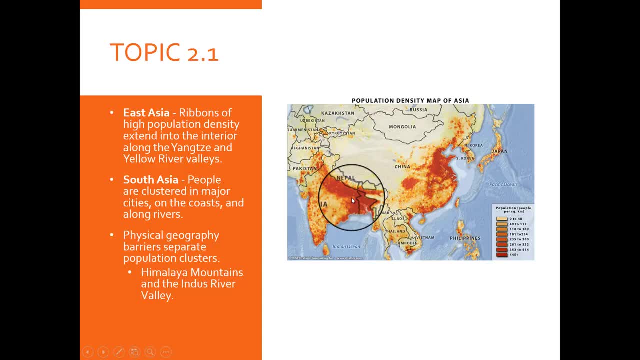 Okay, And they, a lot of the population, started around the areas. you know ancient wise along, you know rivers and valleys and so forth that helped to draw water Right. So in East Asia, here we have the Yangtze River and the Yellow Rivers that helped to. 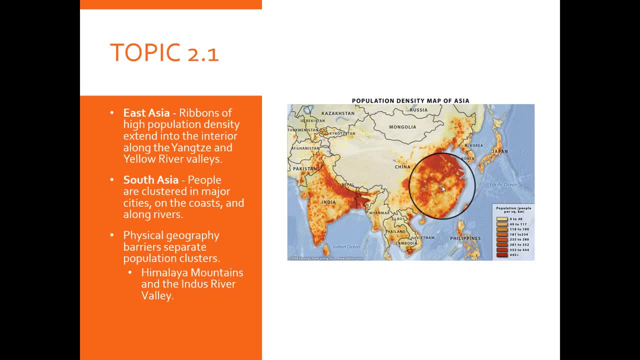 provide water and food Right. In South Asia, which is India and so forth, major people just clustered around major cities, around the coast and along the rivers, so that they can get food, Okay. However, there are physical barriers, Populations such as mountains and maybe other valleys and canyons or something like that. 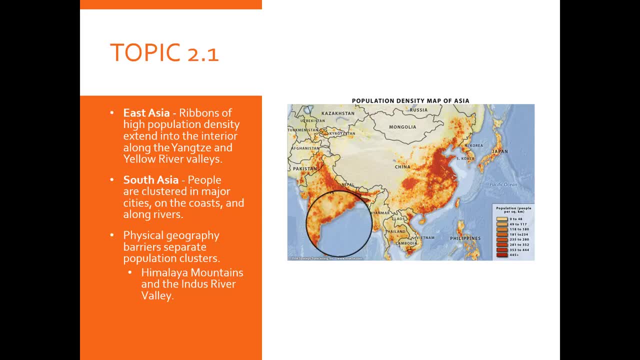 that would separate populations and create physical barriers between populations So they may not thrive as much. So in this case, if you look at this map, the Himalayan Mountains, which is a region right here, kind of makes that separation between the clusters or the concentration. 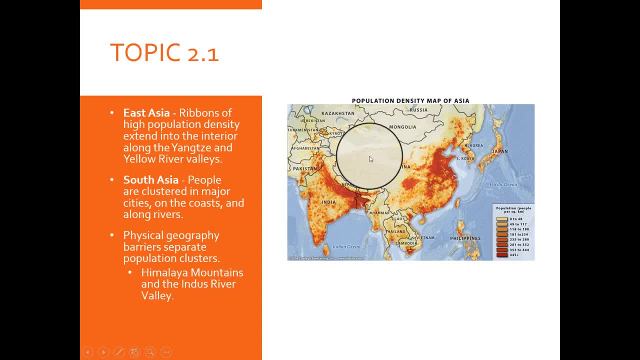 of the population in certain areas. There's not much here, but there's a lot. there's a lot here, Right, Because number one is close to the ocean and two, the Himalayan Mountains, is kind of making that that barrier of having living in this area. 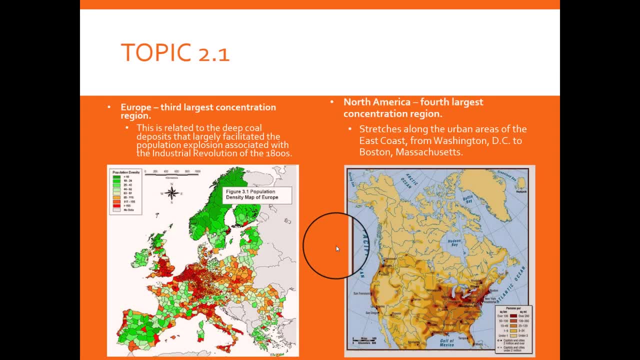 Right, All right. So Europe is the third largest concentration And because this is related to the deep coal deposits that happen, or they they're used during that time And that helped to explode or to help to develop Europe during the Industrial Revolution. 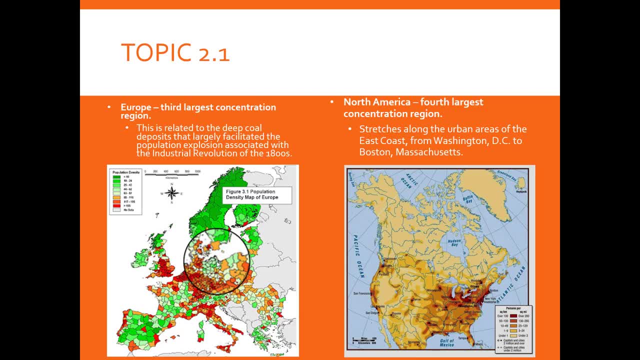 in the 1800s. So the more that they were able to use that coal to fuel things like the steam engine and to help build massive industrial buildings and so forth, to help them with textiles and cloths and other types of resources that we use on a daily basis. 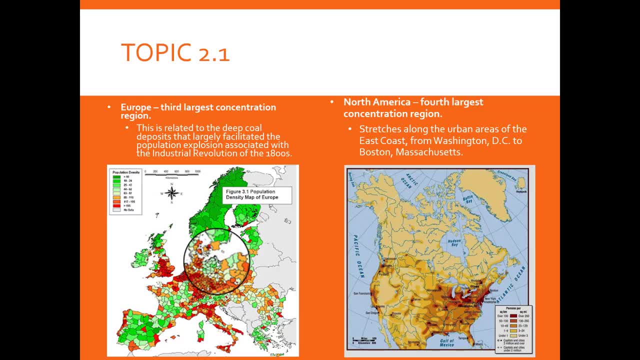 That's how Europe was able to really escalate in its population and also have a high concentration of people, as you see here in the map Right. Then fourth, of course, is North America, And a lot of the urban areas stretch from the east coast to mostly on the east coast. 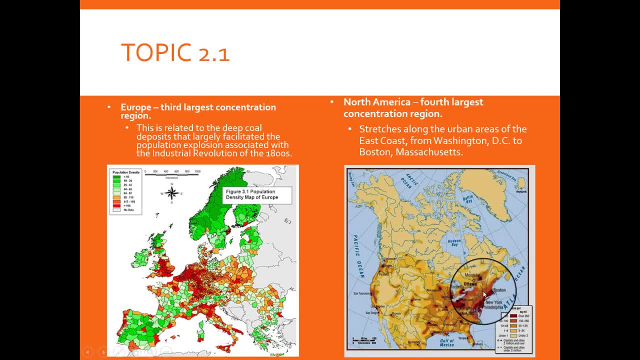 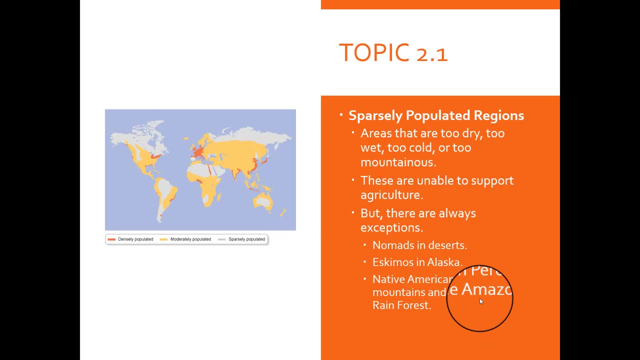 So from Washington DC and in the Boston area, and, of course, you know, New York City has a lot of high concentration, A high concentration of people, Right, All right. However, there are places that are sparsely populated. 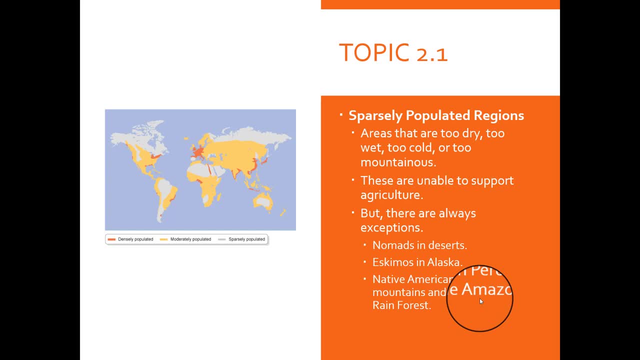 So before we talked about densely populated. So population density where there's a certain concentration of people in certain places on earth, Right. But however, there are places that are sparsely populated, meaning that there's not much people there. 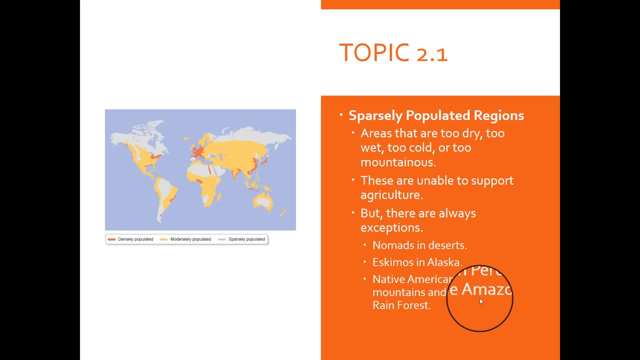 And the reason why there's not much people there is because- number one, it's too dry, There's not enough water. Nobody wants to live where there's no water. Right, Or it's too wet, or it's too cold, or you just can't get there. It's just too mountainous, Right. If there's basically a way not to be able to support any form of food, like agriculture, to grow crops, or we can't get water, then more than likely that's a place that we're not going to live. 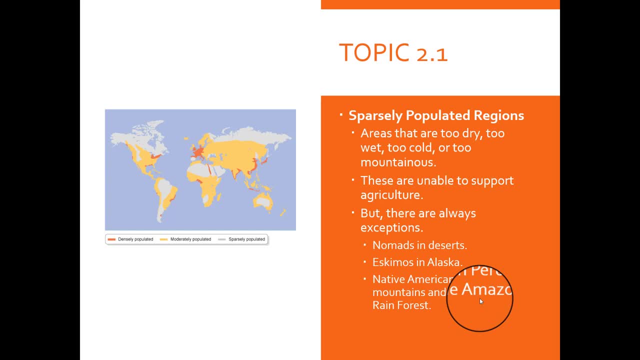 Okay, For example, we're not going to live in Antarctica. It is way too cold. The penguins can have fun there, but not us. Okay, However, that's not always the case. There are some exceptions to this rule, where there's densely populated areas, but then 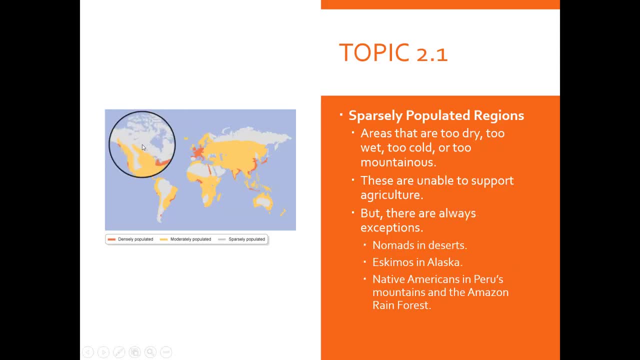 you have the places that are not so populated, like up here in Alaska and the Siberian area, But there are exceptions. So there's nomads that live in the Sahara desert and they adapt as much as they can, or Eskimos that live in Alaska, the Native Americans that live in the Amazon rainforest. 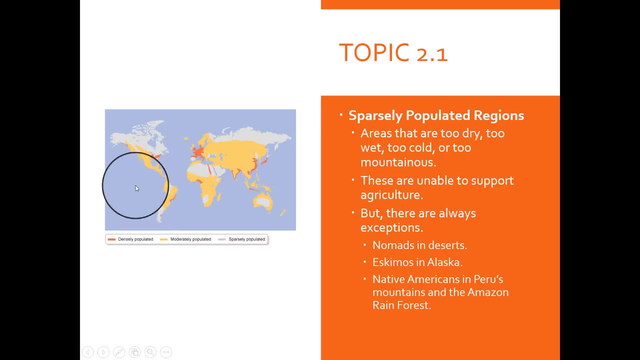 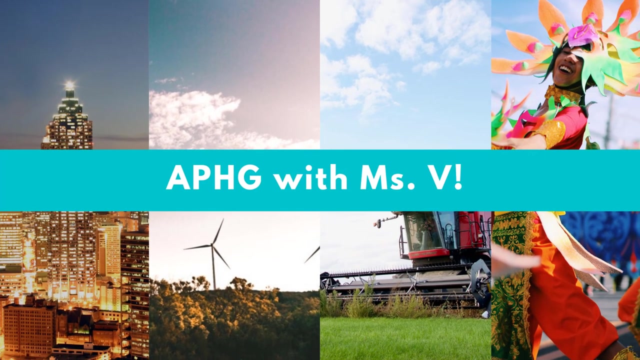 in here in these areas. So they figured out a way to kind of adapt to their environment, Right, A little bit of possible-ism. So if you remember that from the last unit that's incorporating that term, Right, Hey. so I know this is a lot to chomp on, so take a few minutes, get a break.